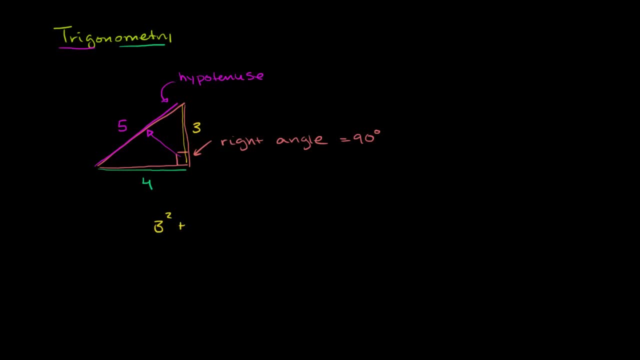 that 3 squared plus 4 squared has got to be equal to the length of the longest side. The length of the hypotenuse squared is equal to 5 squared, So you can verify that this works out. This satisfies the Pythagorean theorem. 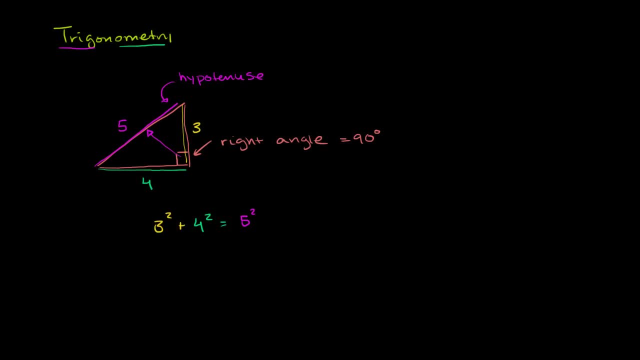 Now, with that out of the way, let's learn a little bit of trigonometry, So the core functions of trigonometry. we're going to learn a little bit more about what these functions mean. There is the sine function, There is the cosine function. 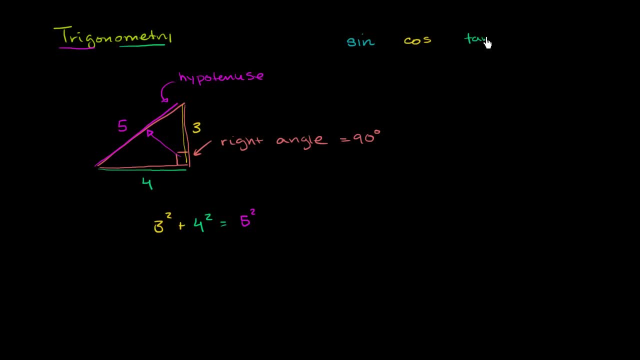 And there is the tangent function And you write sin, cos or S-I-N, C-O-S and tan for short, And these really just specify for any angle in this triangle it'll specify the ratios of certain sides. So let me just write something out. 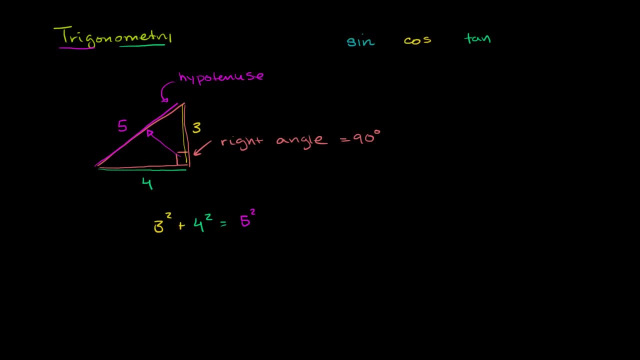 And this is a little bit of a mnemonic here, so something just to help you remember the definitions of these functions. But I'm going to write down something. It's called SOH-CAH-TOA and you'll be amazed how far this mnemonic will take you in trigonometry. 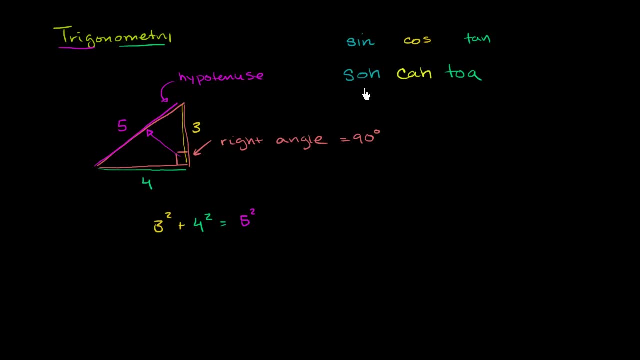 So we have SOH-CAH-TOA, And what this tells us is that sine is equal to opposite over hypotenuse. It's telling us- And this won't make a lot of sense just yet. I'll do it in a little bit more detail in a second. 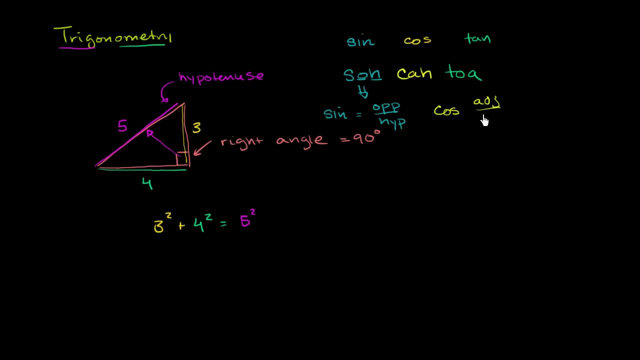 And then cosine is equal to adjacent over hypotenuse, Cosine is equal to adjacent over hypotenuse, And then you finally have tangent. You have tangent is equal to opposite over adjacent. So you're probably saying, hey, Sal, what is all this? opposite, hypotenuse, adjacent. 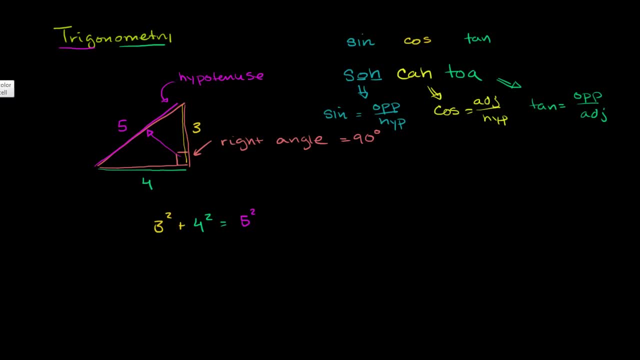 What are we talking about? Well, let's take an angle here. Let's take an angle here. Let's say that this angle right over here is theta, between the side of length 4 and the side of length 5.. This angle right here is theta. 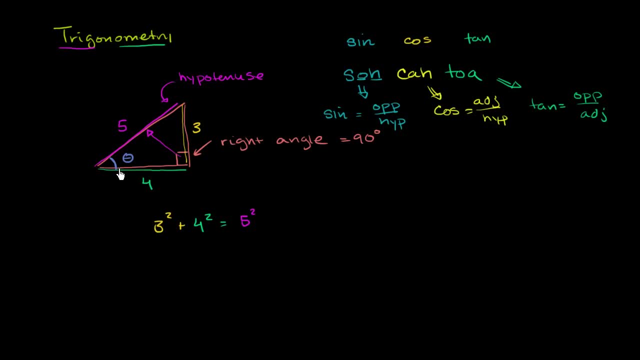 So let's figure out what the sine of theta, the cosine of theta and what the tangent of theta are. So if we want to first focus on the sine of theta, we just have to remember SOH-CAH-TOA. 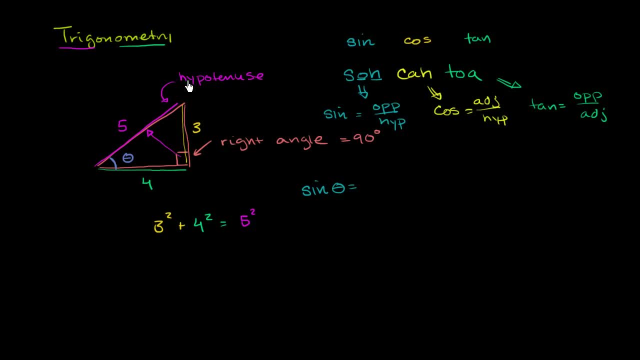 Sine is opposite over hypotenuse. so sine of theta is equal to adjacent over hypotenuse. The opposite. So what's the opposite side to the angle? So this is our angle right here, The opposite side, the opposite side. 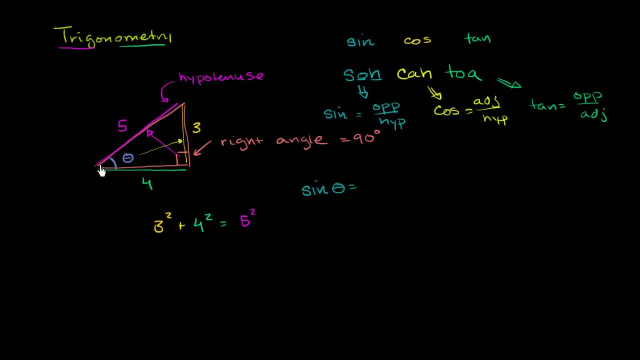 if you just go the opposite side, so not one of the sides that are kind of adjacent to the angle, the opposite side is the 3. If you're just kind of, it's opening on to that 3.. So the opposite side is 3.. 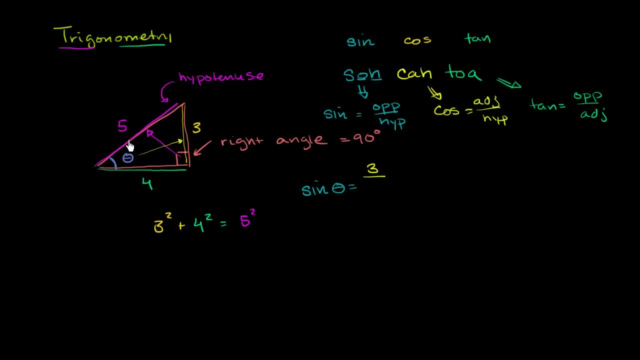 And then what's the hypotenuse? Well, we already know: the hypotenuse here is 5.. So it's 3 over 5.. The sine of theta is 3 fifths. So someone says, hey, what's the sine of that? 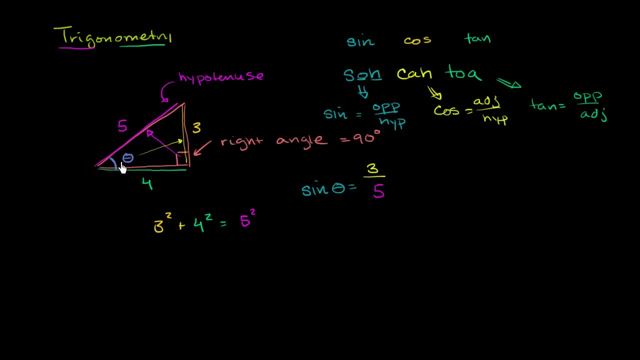 It's 3 fifths And I'm going to show you in a second that the sine of theta, if this angle is a certain angle, it's always going to be 3 fifths, The ratio of the opposite to the hypotenuse. 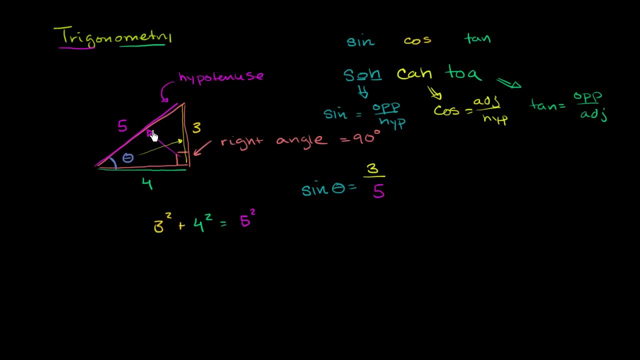 is always going to be the same, even if the actual triangle were a larger triangle or a smaller one. So I'll show you that in a second. But let's go through all of the trig functions. Let's think about what the cosine of theta is. 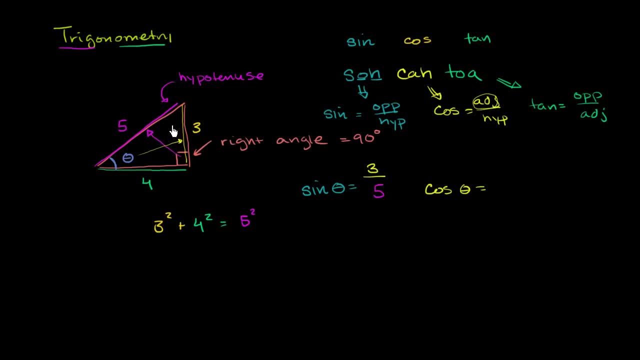 Cosine is adjacent over hypotenuse. So remember, let me label them. We already figured out that the 3 was the opposite side. This is the opposite side, And only when we're talking about this angle. When you talk about this angle, this side is opposite to it. 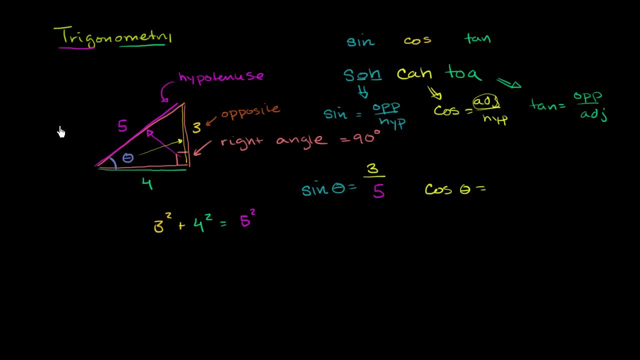 When you talk about this angle, this 4 side is adjacent to it. It's one of the sides that kind of make up that kind of form, the vertex here. So this right here is an adjacent side, And I want to be very clear. 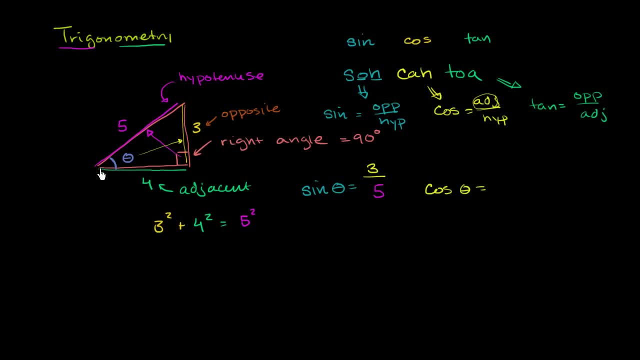 This only applies to this angle. If we were talking about that angle, then this green side would be opposite and this yellow side would be adjacent, But we're just focusing on this angle right over here. So cosine of this angle we hear about adjacent. 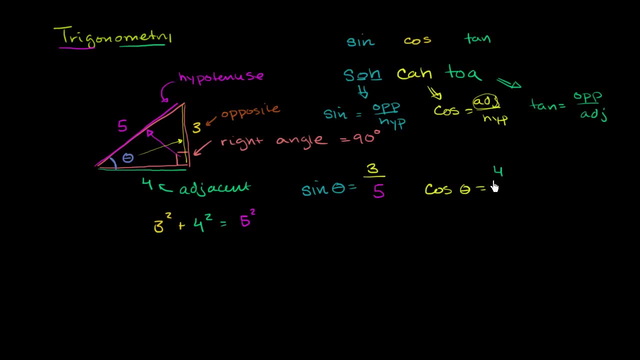 Well, the adjacent side of this angle is 4.. So it is adjacent over the hypotenuse. It's the adjacent which is 4, over the hypotenuse, 4 over 5.. Now let's do the tangent. 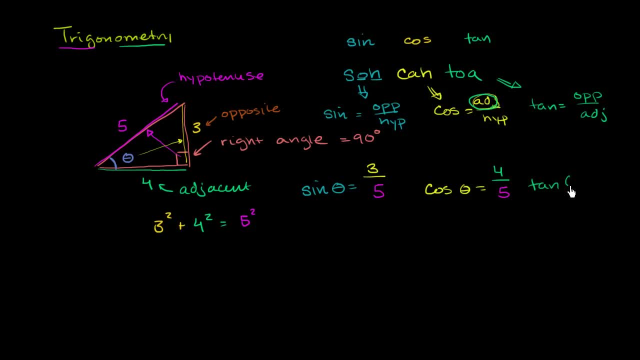 Let's do the tangent, The tangent of 4.. Let's do the tangent of theta: Opposite over adjacent. The opposite side is 3.. The opposite side is 3.. What is the adjacent side? We already figured that out. 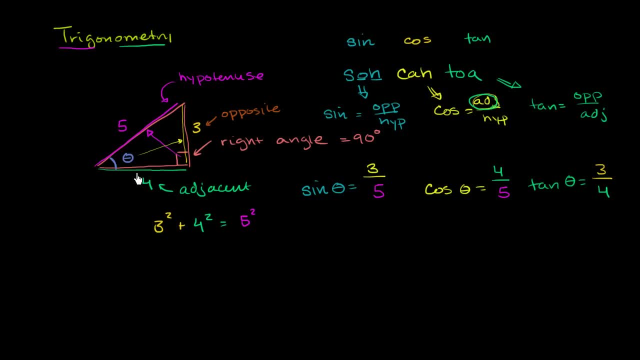 The adjacent side is 4.. So, knowing the sides of this right triangle, we were able to figure out the major trig ratios. And we'll see there are other trig ratios, but they can all be derived from these 3 basic trig functions. 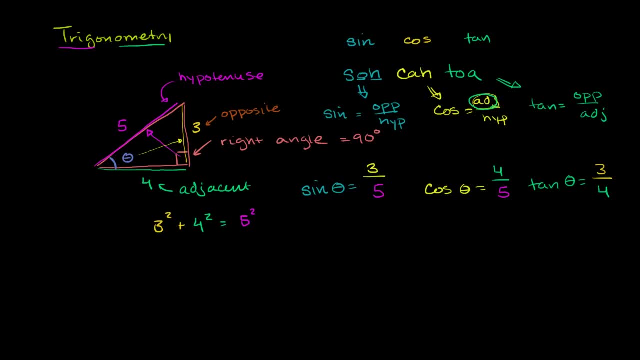 Now let's think about another angle in this triangle, And I'll redraw it Just because my triangle is getting a little bit messy. So let's redraw the exact same triangle, The exact same triangle, And once again, the lengths of this triangle are: 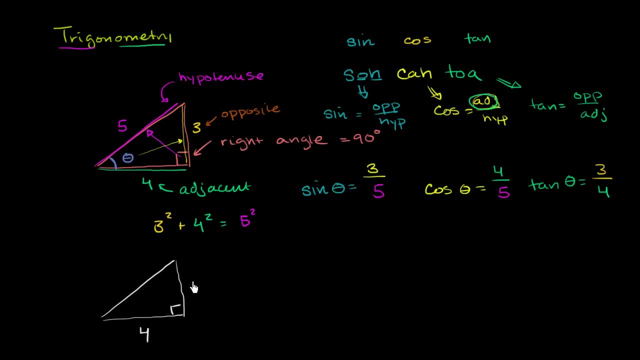 we have length 4 there, We have length 3 there, We have length 5 there. The last example: we just we used this theta, But let's do, let's do another angle, let's do another angle up here. 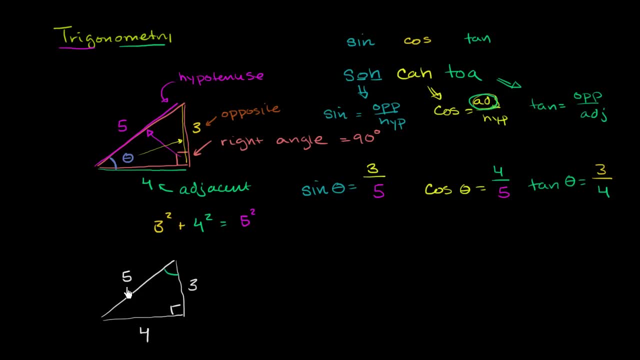 Let's do another angle up here And let's call this angle- I don't know, I'll think of something- a random Greek letter. So let's say it's xi. I know it's a little bit bizarre. Theta is what you normally use. 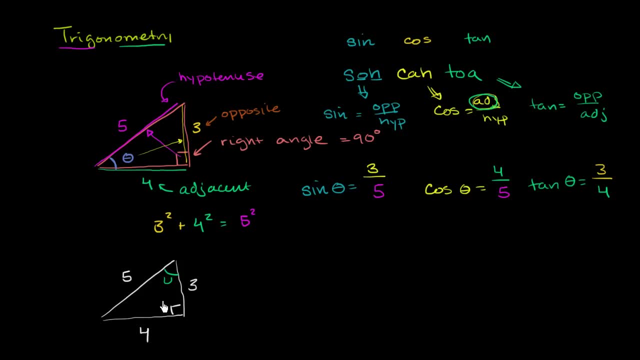 but since I already used theta, let's use xi Actually instead of xi. let me just simplify it. Let me call this angle x, Let's call that angle x. So let's figure out the trig functions for that angle x. 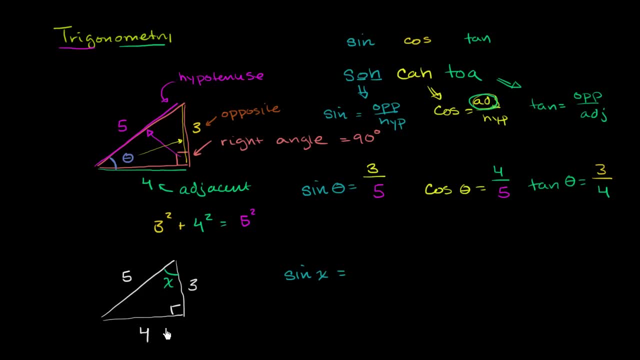 So we have: sine of x is going to be equal to what? Well, sine is opposite over hypotenuse. So what side is opposite to x? Well, it opens onto this triangle. This is 4.. It opens onto the 4.. 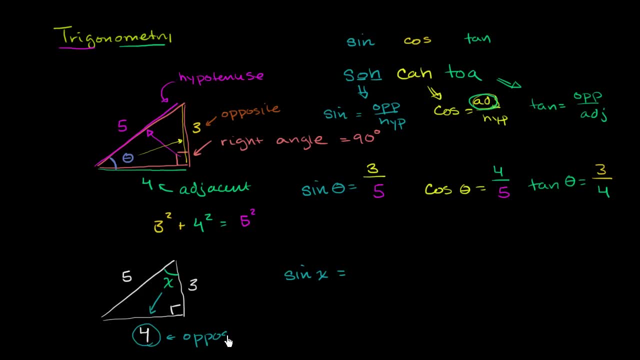 So, in this context, this is now the opposite. This is now the opposite side. Remember, 4 was adjacent to this theta, but it's opposite to x, So it's going to be 4 over now. what's the hypotenuse? 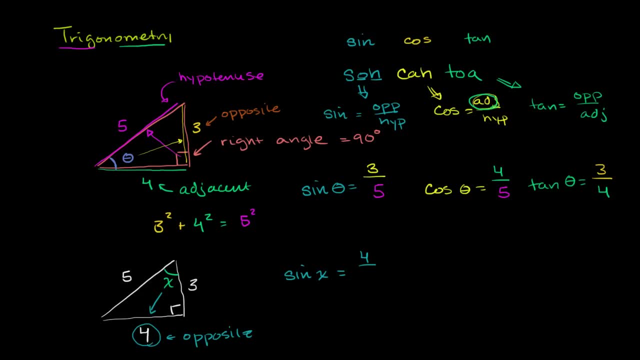 Well, the hypotenuse is going to be the same regardless of which angle you pick. So the hypotenuse is now going to be 5.. So it's 4. fifths, Now let's do another one. What is the cosine?